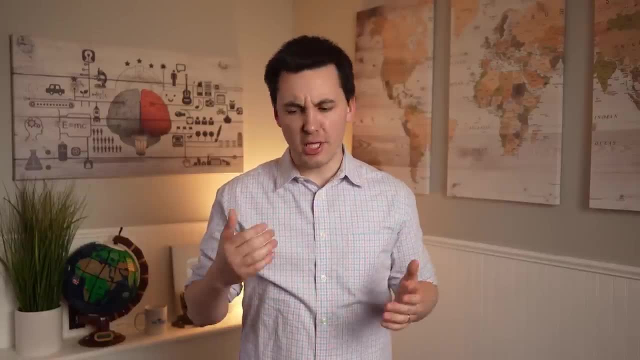 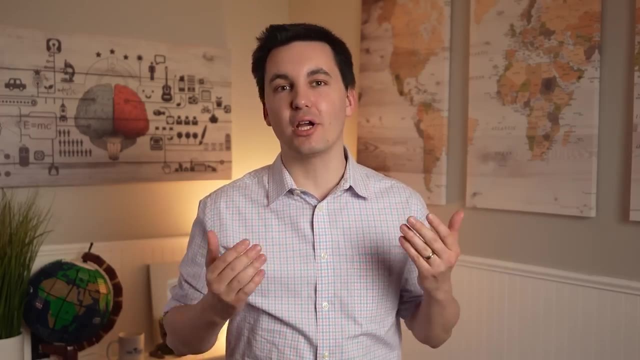 regulated or protected by the government. Jobs and activities in the informal economy often do not have access to formal financial services. they lack consistent income and often do not have regulations or legal protections. Jobs such as street vendors, domestic work, illegal businesses or events that are illegal are dealt with by the government. The economic 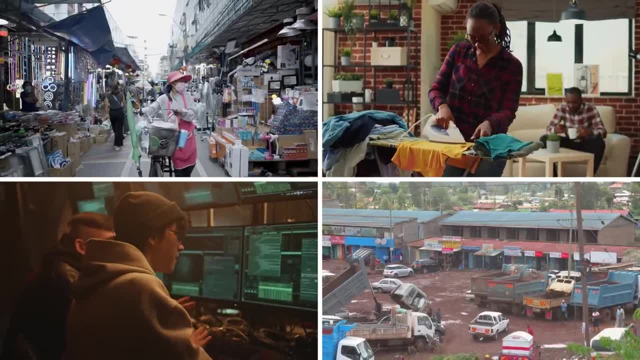 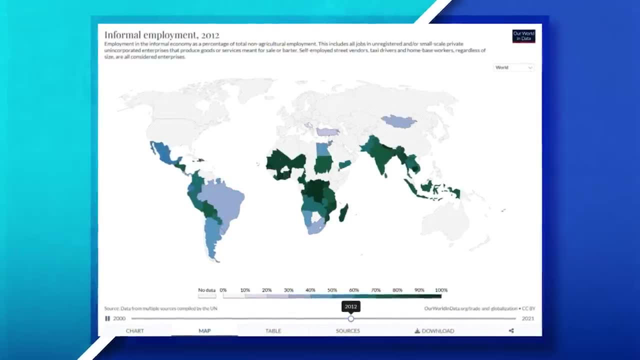 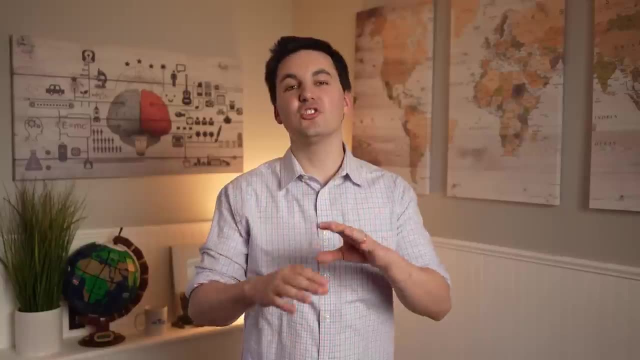 businesses or unregistered small businesses would all be examples of jobs in the informal economy. Traditionally, we can see that countries that have less economic development generally have a significant amount of jobs and activities located in the informal economy instead of the formal economy. Now, since the informal economy is not regulated or overseen by the government, it can be difficult. 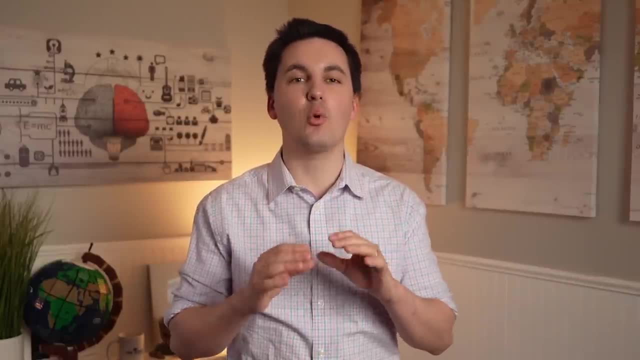 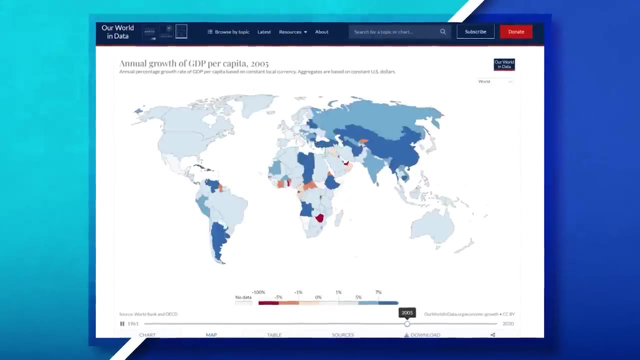 to measure. However, we can measure the formal economy in a variety of different ways. The first measure we can use is the GDP, which stands for Gross Domestic Product. This measures the total economic output of a country over a given period of time. 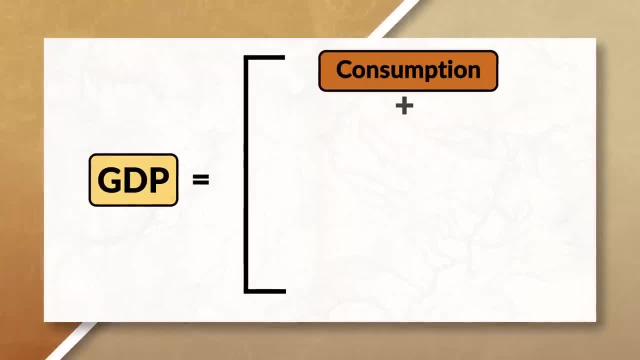 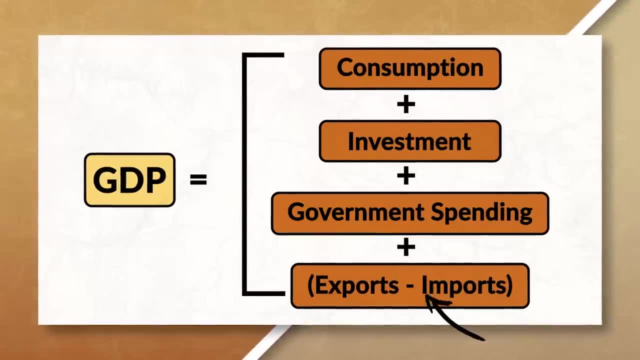 We can get a country's GDP by adding a country's consumption, investment, government spending and the country's exports minus its imports. Notice that we are subtracting imports from our calculation. This is because the GDP is only factoring in production that occurs inside the country's. 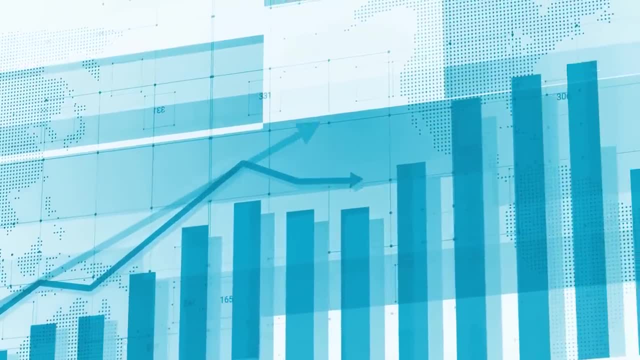 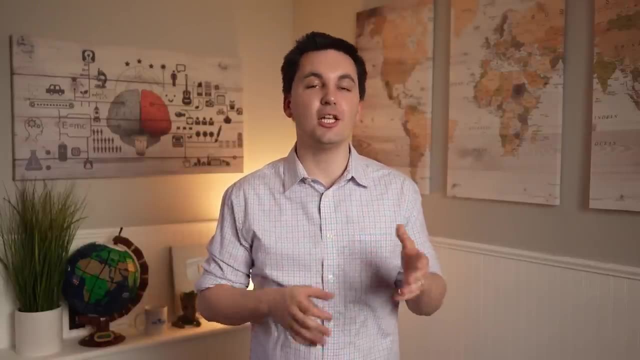 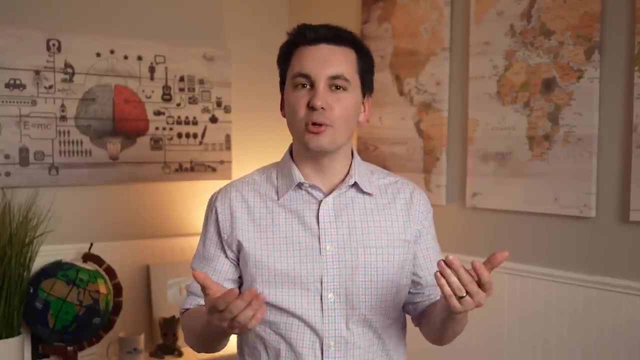 boundaries. When GDP is increasing, it shows that businesses are expanding, Jobs are being created and the economy is growing. We can also see that when the GDP is increasing, it indicates that there is more consumer and government spending, which is due to the government receiving more tax revenue and consumers having 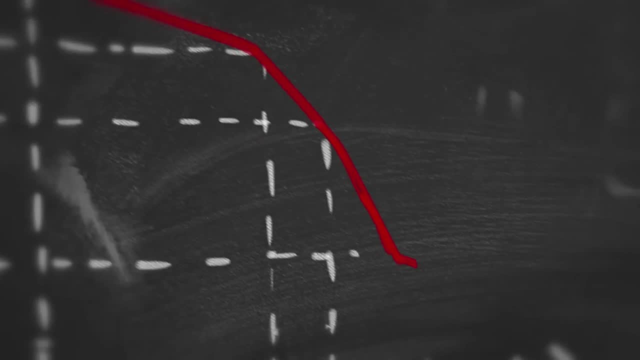 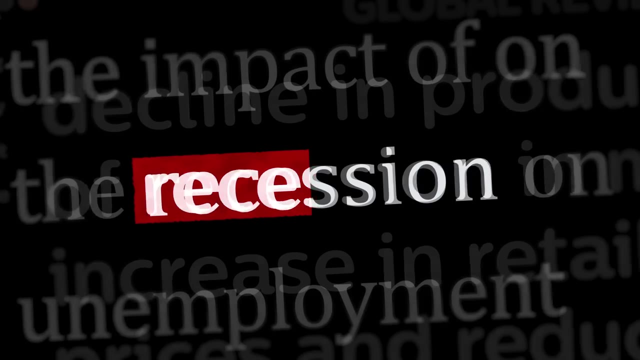 more disposable income, But, on the other hand, when GDP is declining, it shows that the total value of goods and services inside the country's boundaries is shrinking, which can be due to the result of an economic contraction or possibly a recession. A decrease in the GDP also often indicates that businesses are expanding. 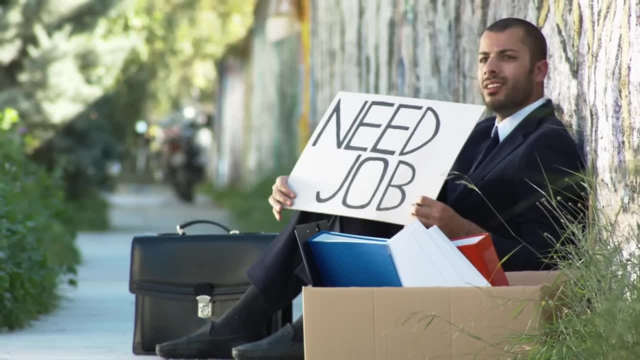 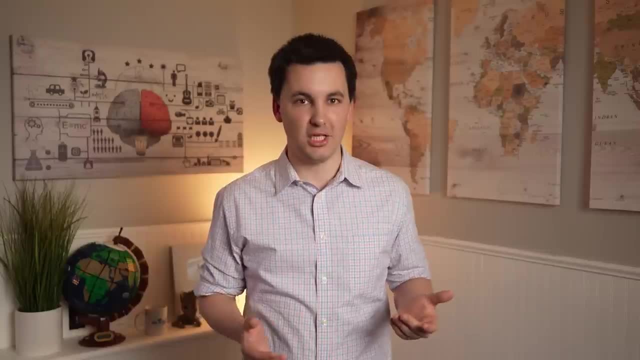 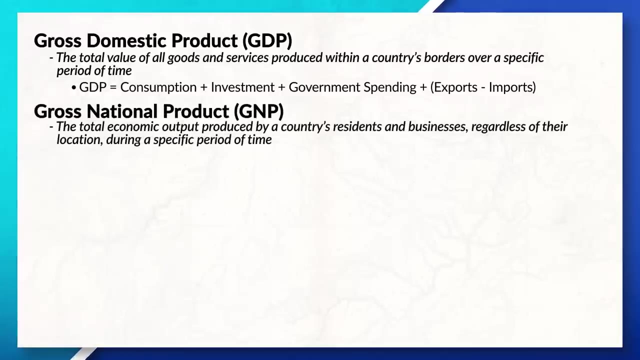 This indicates that businesses may be struggling, that jobs are being lost and that consumers are spending less money. Another way in which we can observe economic development is by looking at the GNP, which stands for the Gross National Product. The GNP includes the value of all goods and services produced by a country's citizens. 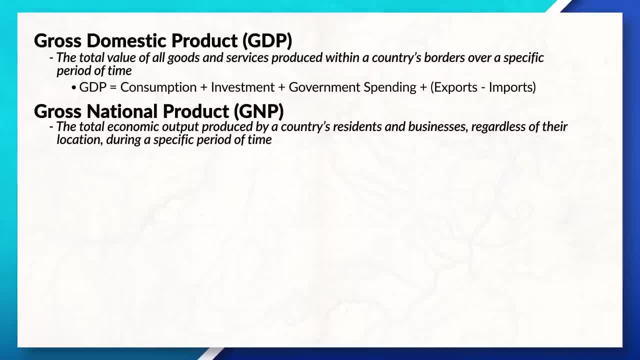 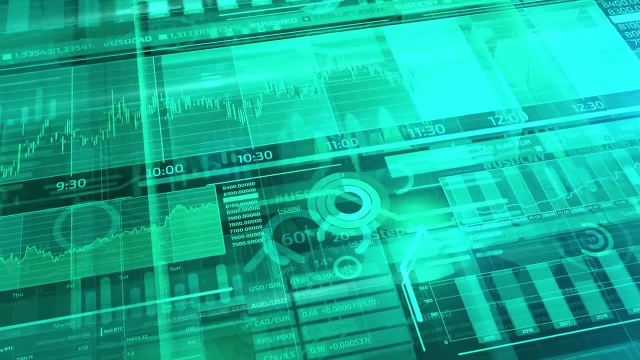 regardless of where they are located in the world. Both the GNP and GDP are pretty similar. However, the key difference is the GNP factors in both domestic production and the production of citizens who are living abroad. Remember, the GNP is only looking at the production of goods and services by the nationality of. 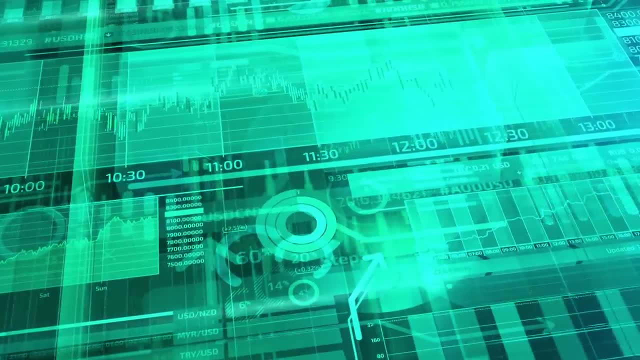 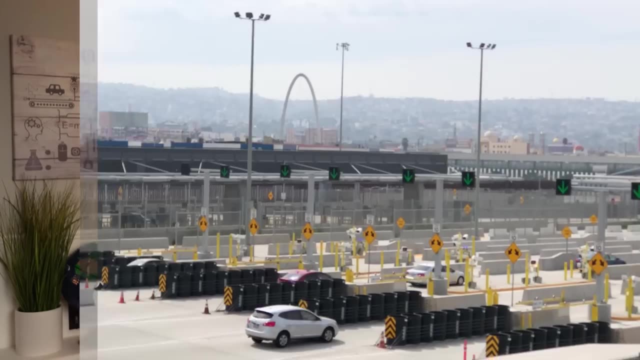 the country, so any foreign production inside the country's boundaries would not count for the GNP. If a country's GNP is larger than its GDP, it can mean a couple of different things. It could be that there is a significant amount of citizens living abroad and no longer living. 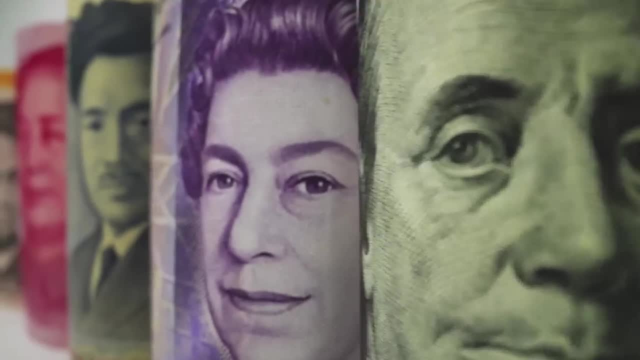 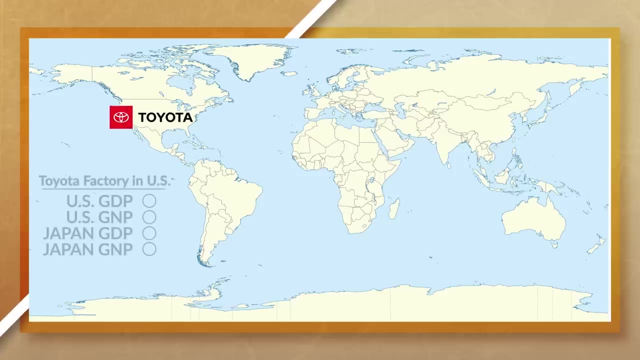 inside the country's boundaries. Or it could also mean that there is a lot of foreign investment and production happening inside the country's boundaries. To better illustrate these two concepts, think of it this way: If Toyota builds a factory in the United States to produce cars in the country, that is part 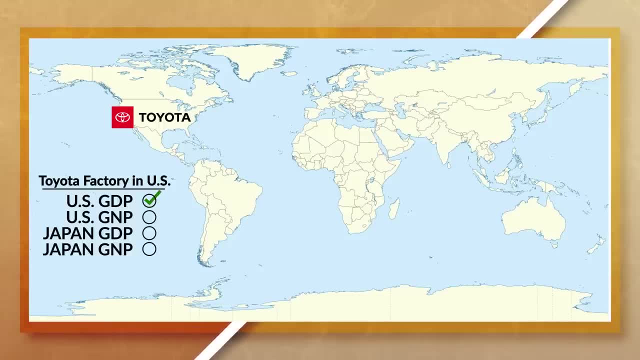 of the United States' GDP, since production is happening domestically in the United States. However, Toyota is not a US-based company, so this production would not be part of the United States' GNP and instead would be part of Japan's GNP, since Toyota is a Japanese. 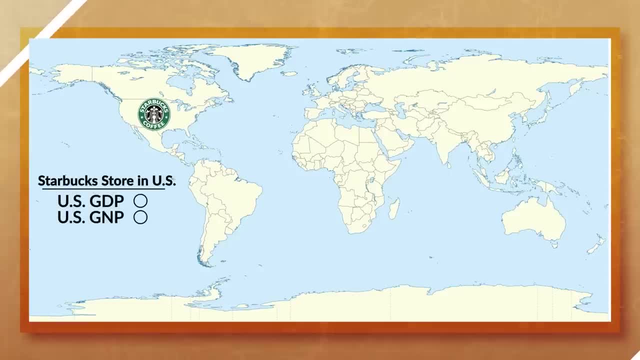 company. Or take Starbucks, for example. When they open a new store inside the United States, it is part of the United States' GNP. But if Starbucks opens stores in China, those stores would be part of China's GDP and not. 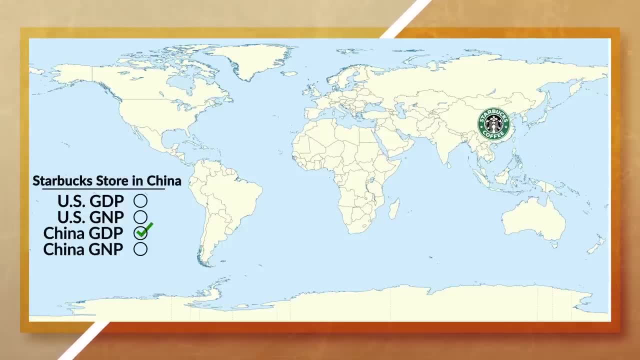 the United States' GDP, since the production is occurring inside China's boundaries. But remember, Starbucks is still an American company, so it would be part of the United States' GNP and not China's. Up next, we have the GNI, which stands for Gross National Income. 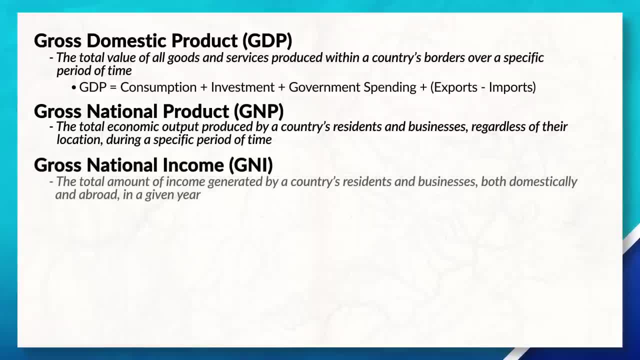 To calculate the GNI, you need to add up the income generated by all of the country's citizens, regardless of whether or not you are a Chinese citizen or not. The GNI stands for Gross National Income. This would include wages, profits and also investments. 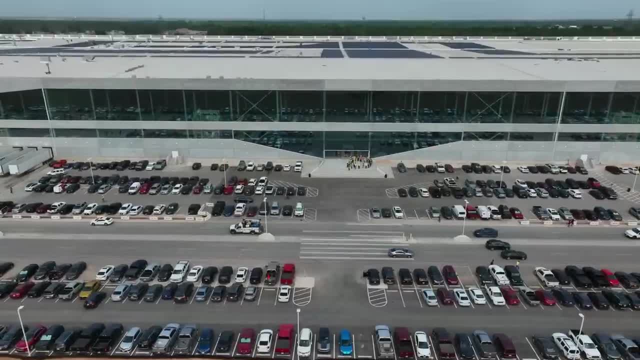 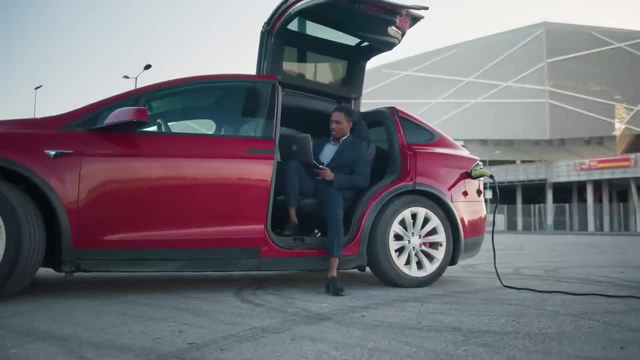 Notice here, the focus is on income, not production. For example, Tesla is an American-based company, but has factories in countries around the world and earns profits from the sale of goods produced in those factories. If we were looking at the GDP of the United States, we would only factor in the production. 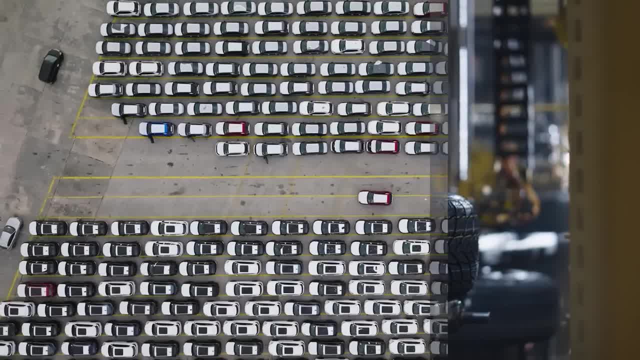 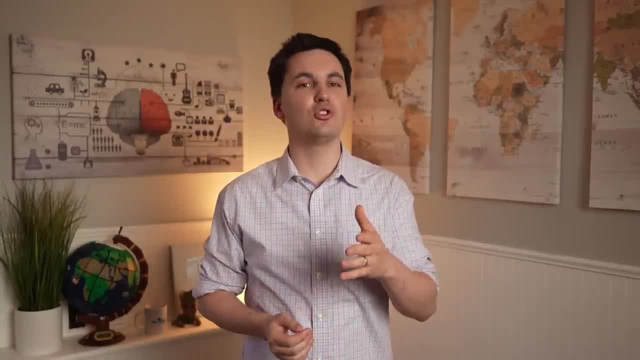 of the Tesla sales inside the United States' boundaries. but when looking at the GNI, we would also include the profit from the GNI. Now you might be thinking: how does this differ from a country's GMP? And to be fair, it's a great question. 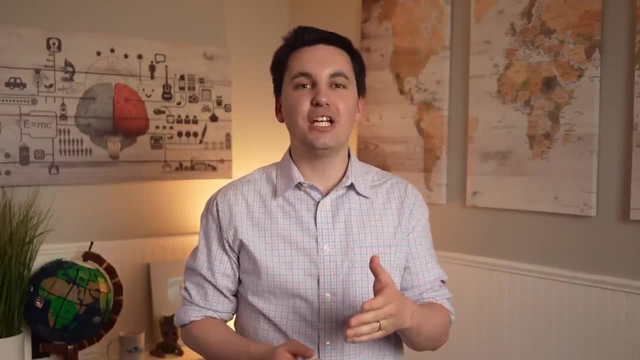 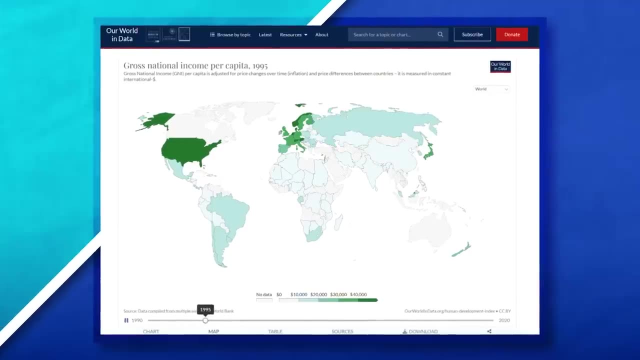 The main difference between the GNI and the GMP is: the GNI focuses on income generated by a country's citizens and companies, while the GMP focuses on production. We can also look at the GNI per capita, which is often used as a way to better understand. 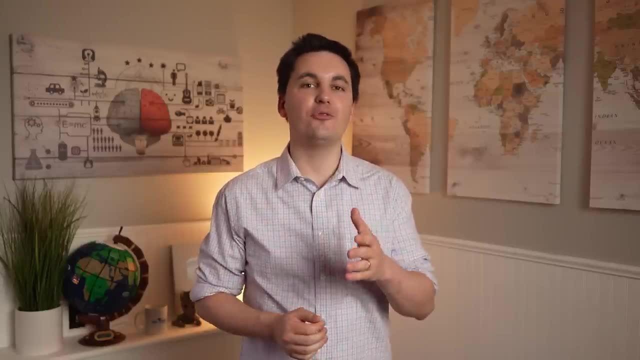 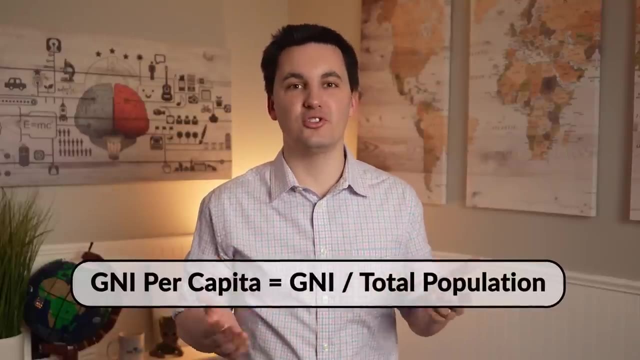 a country's standard of living. To find the GNI per capita, we have to take a country's GNI and divide it by its population. Remember, the GNI includes the GNI per capita. The GNI includes the total income earned by a country's citizens. 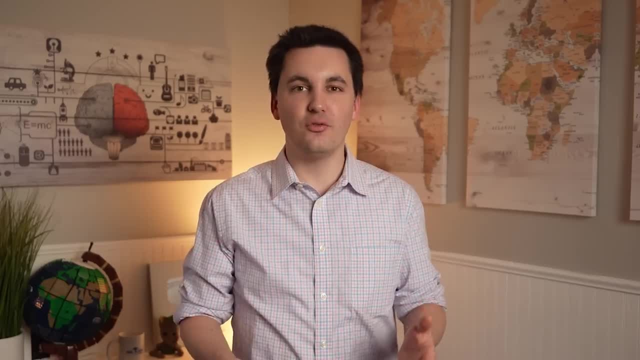 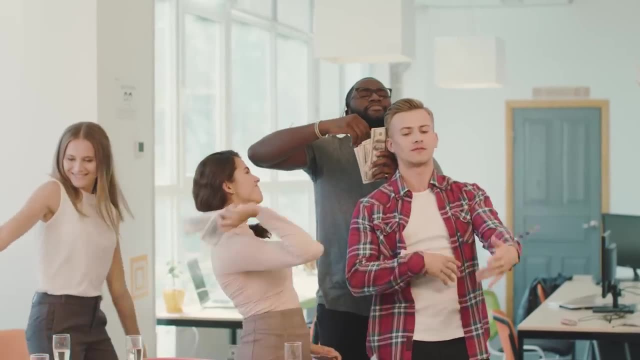 This includes all wages, profits and investments, both by individuals and businesses. So the GNI per capita allows us to gain an estimate that shows us the average income earned by each person in the country. Generally, the higher the GNI per capita, the more economic opportunities there are. 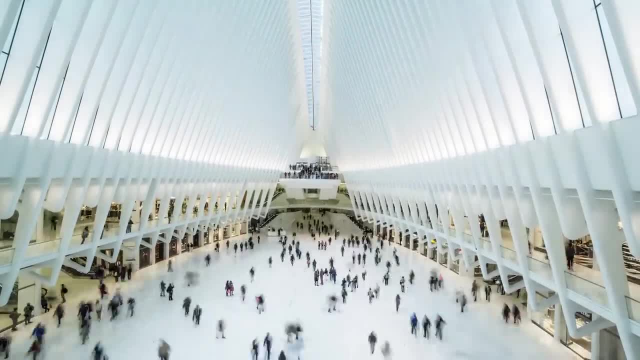 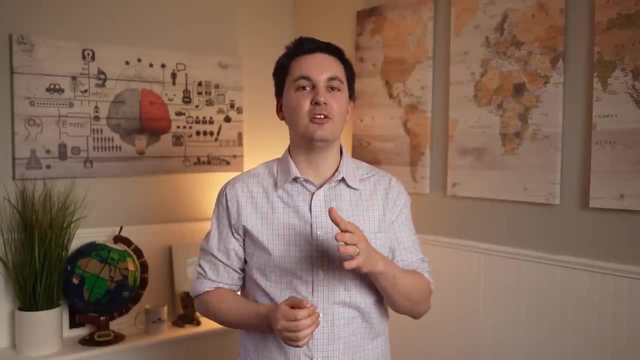 in society, along with the more goods and services that people have access to And the higher the standard of living is. one thing to note is that the GNI per capita does not show income inequality, quality of life or other social aspects, so it does. 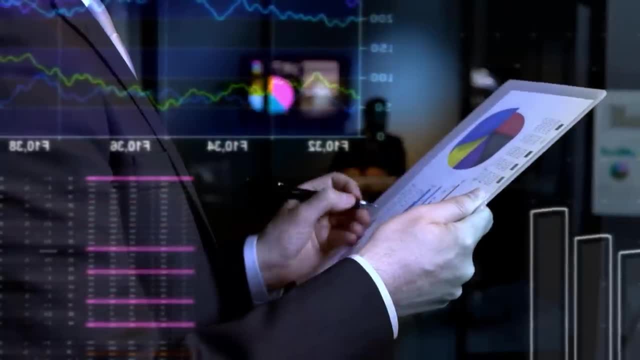 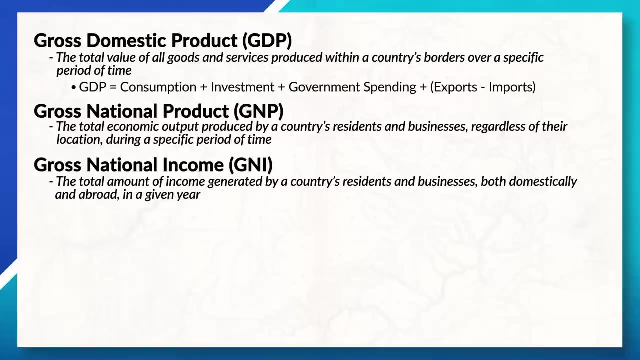 not show an entire picture of a country. Now, so far, we've been looking at ways in which we can measure economic development of a country, but we can also measure a country's social development as well. One way we can do this is by looking at a country's GII, which is the Gender Inequality. 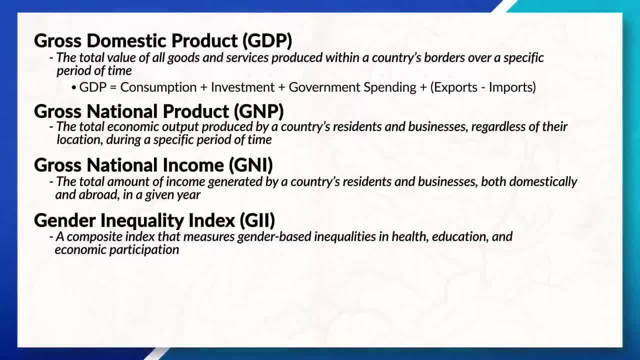 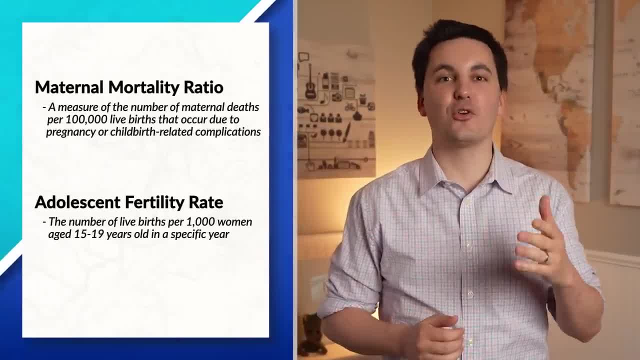 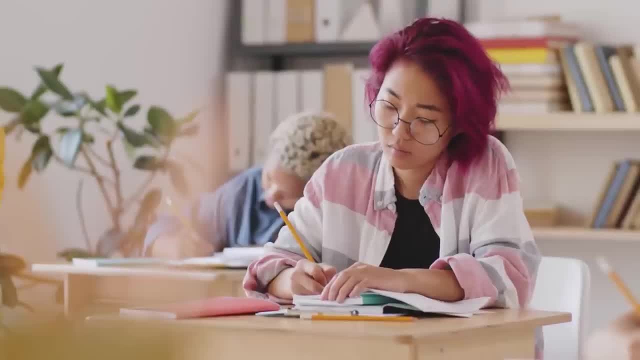 Reproductive health, empowerment and the labor market, The national mortality ratio and the adolescent fertility rate. Empowerment is measured by the amount of government positions held by each gender and the amount of secondary and higher education levels obtained by each gender. 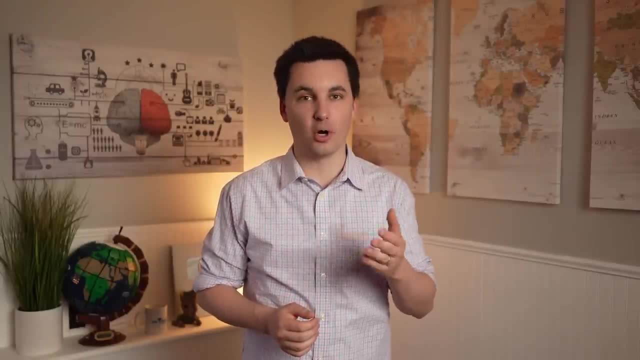 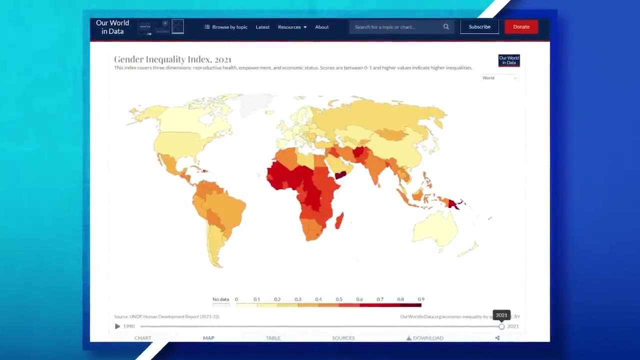 Lastly, the labor market is measured by women's participation in the workforce. A country's GII can range between 0 and 1, with the higher values indicating more inequalities and disparities between women and men. If the GII for a country is ever 0,, it would mean there is no inequalities in society. 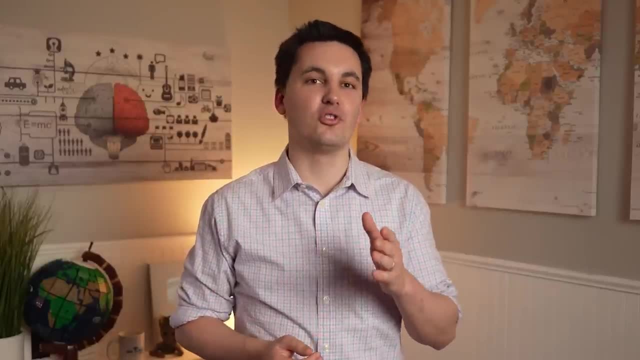 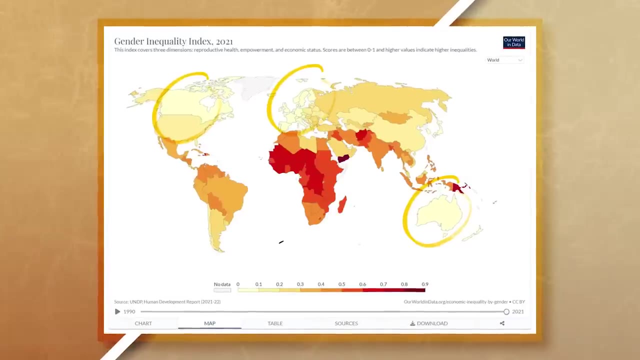 and the country has perfect equality. Currently, however, there are no countries in the world with a score of 0. Notice that generally, we can see that countries that have more economic development are more likely to have a lower GII, while countries that have less economic development generally. 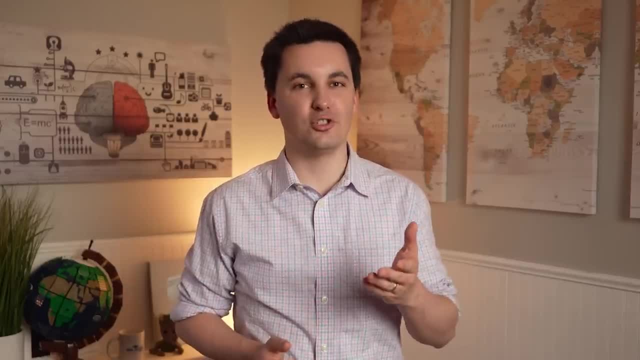 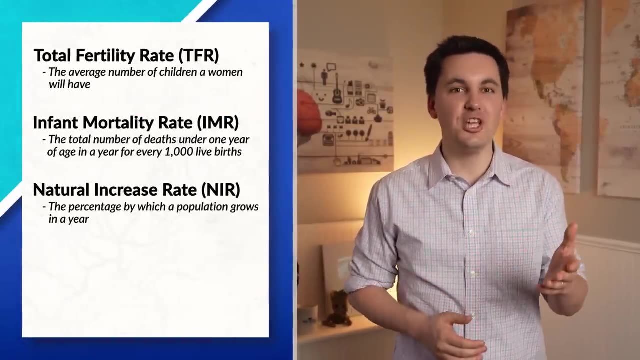 have a higher GII. Here we can also connect back to our Unit 2, where we looked at countries' demographic data and analyzed the impact that economic development has on a country's TFR, IMR literacy rates, access to medicine and population. 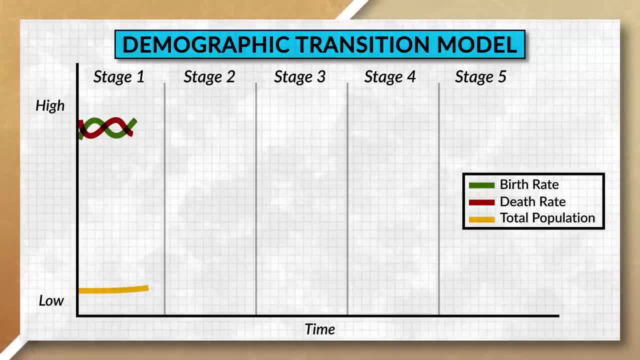 We can also see that countries that have more economic development are more likely to have a lower GII, while countries that have less economic development are more likely to have a higher TFR. Remember, countries that are not far along in the demographic transition model tend to. 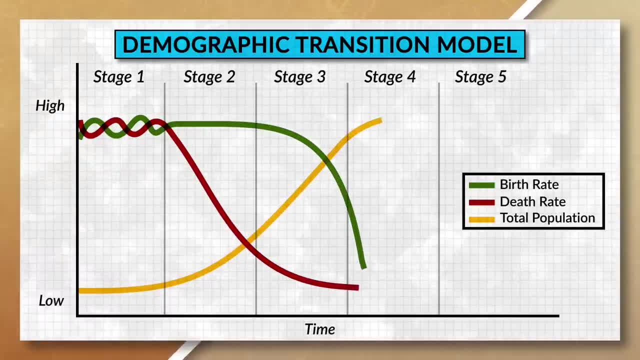 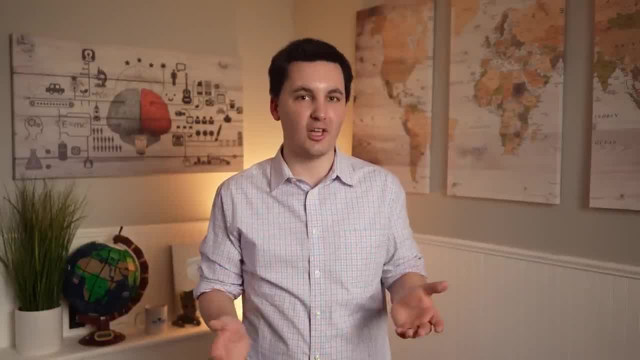 have a high natural increase rate, higher infant mortality rate and higher total fertility rate. They also are more likely to give women less economic and social opportunities in society and have traditional gender roles in place. Now the last indicator we are going to look at is the HDI, which stands for the Human 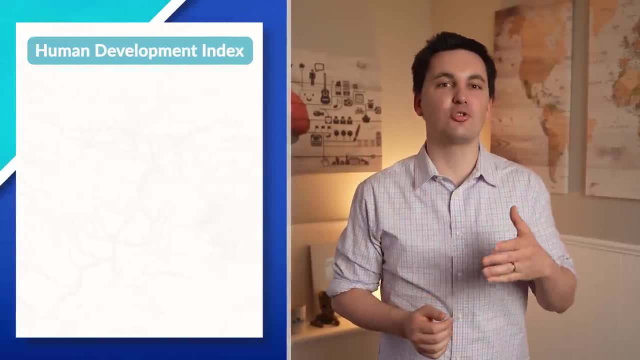 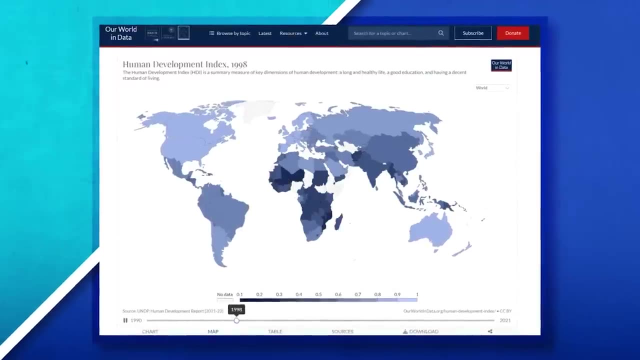 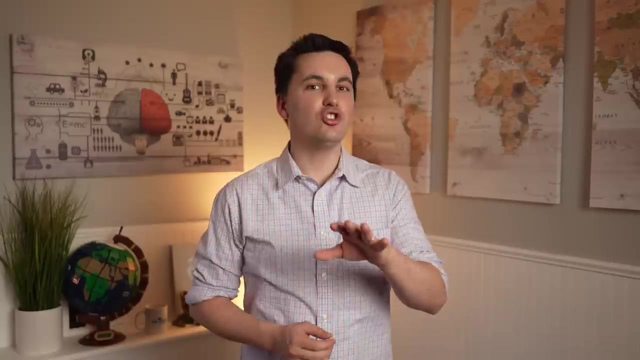 Development Index. This index is determined by looking at a country's life expectancy, expected years of schooling and the gross national income per capita. Just like the GII, the HDI can range anywhere from 0 to 1.. However, unlike the GII, the higher the score, the higher the human development. 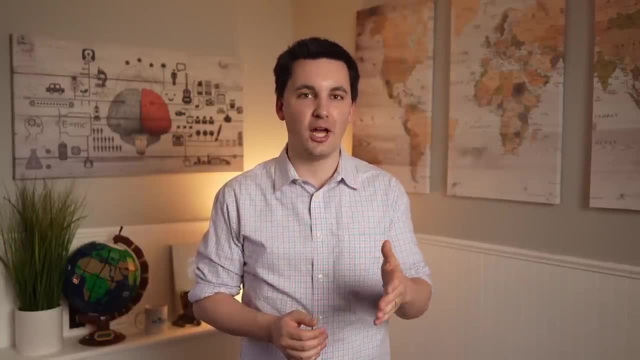 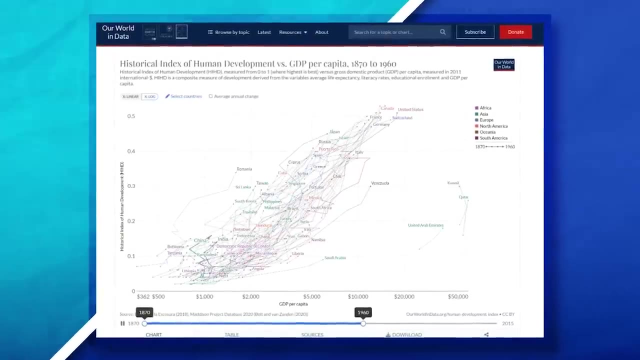 Understanding. the HDI allows us to gain different insights into different countries and compare the level of human development between them. We can also use the HDI to track a country's development over time, to see how a country is developing and identify different areas in which further improvement could occur. 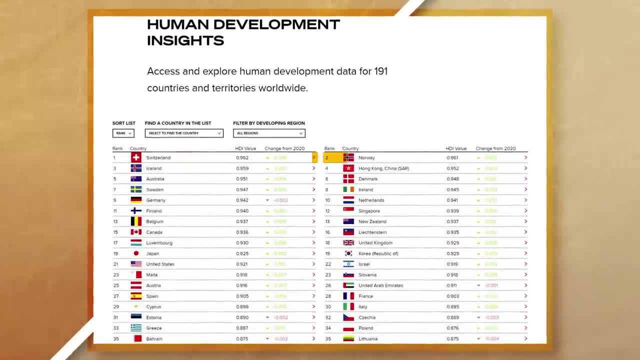 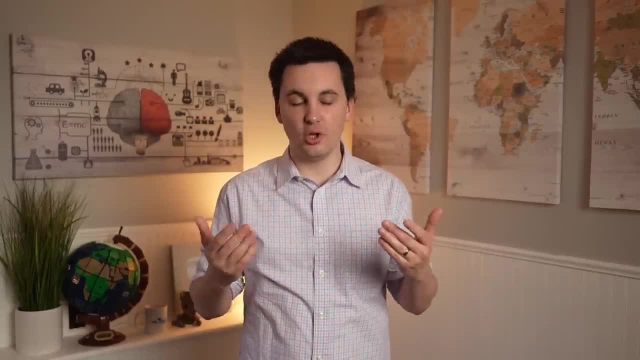 Today, the countries with the highest HDI would be Switzerland, Switzerland, Norway, Iceland, Hong Kong and Australia, just to name a few. One other way in which we can measure development would be to look at the amount of renewable resources and the use of fossil fuels. As countries become more developed, they tend to rely more on fossil fuels to meet their new, growing energy demands. Developed countries are more often more dependent on fossil fuels due to their dependency on cars, planes and other technological advances. Today, though, we are also seeing higher levels of renewable energy be utilized. 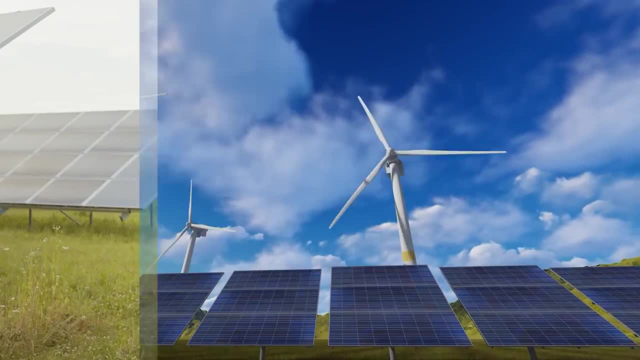 We are also seeing higher levels of renewable energy be utilized in developing countries. We are also seeing higher levels of renewable energy be utilized to help provide energy needs for society. However, once again, it's most commonly found in more developed countries that have access.